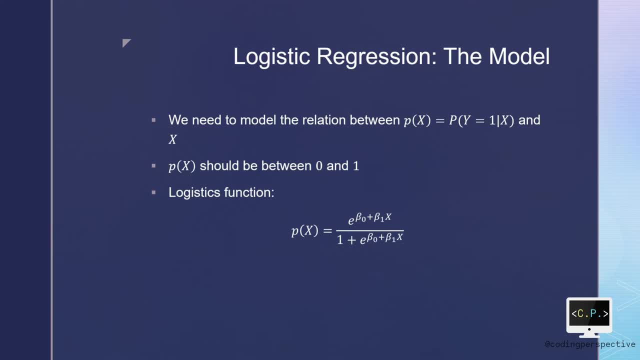 divided by 1 plus e, to the power beta 0 plus beta 1, x. If you think about logistic function, you will see that the function always stays in the range of 0 and 1.. If you think about an example of defaulting, you can consider x as the balance on the customer's account. 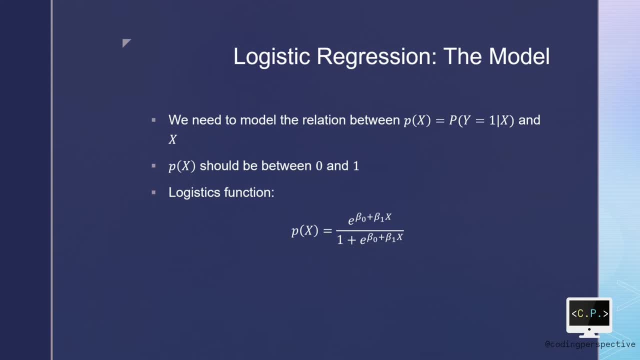 So in that case the prediction of the model will be close to 0.. However, it may never be below 0. So we can also use the logistic function, which is p equal to e to the power beta 0 plus beta 1 x. 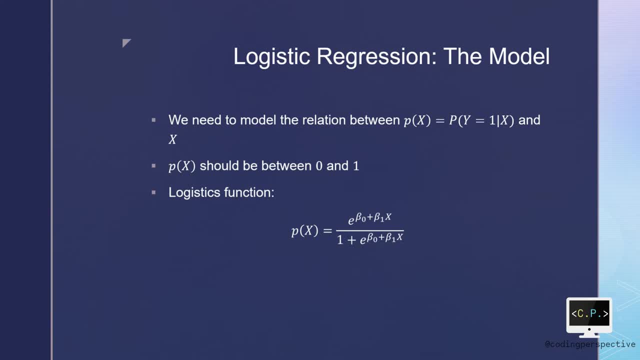 0. because of its construction, The logistic function always creates an s-shaped curve of this form. Regardless of the value of x, we will obtain a sensible prediction. For fitting purposes, we will use the maximum likelihood method, which will be shown in: 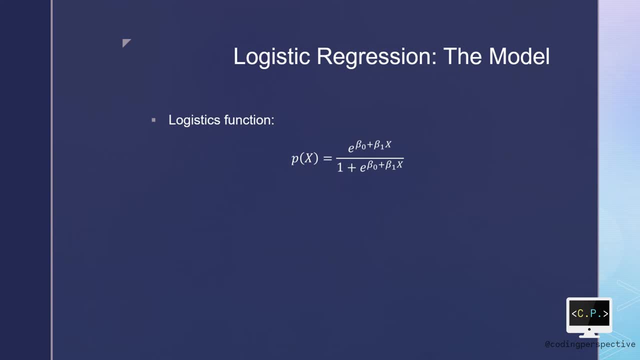 the next slides, Recall the logistics function from the previous slide. What we will do is that we will manipulate a little bit and take the logarithm of both sides where we end up the logistic regression model, That is, the logarithm of px divided. 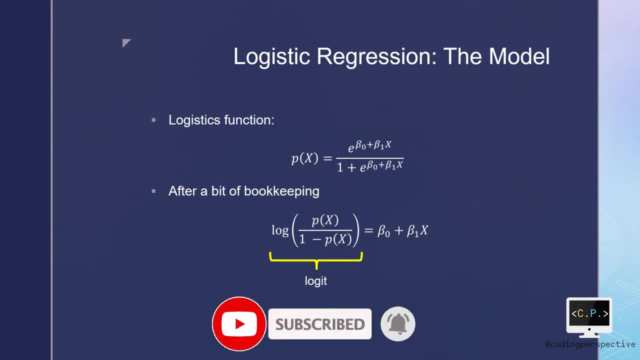 by 1 minus px is equal to beta0 plus beta1x. As you can see on the slide, the logistic regression model is linear in x, which will help us with the interpretability of the model. We will use the maximum likelihood method for estimating beta0 and beta1.. 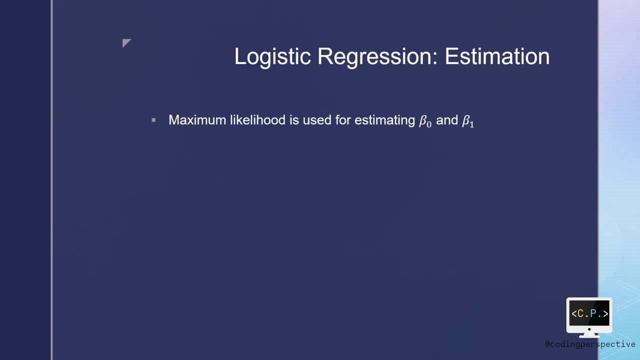 The basic intuition behind using the maximum likelihood method for fitting a logistic regression model is that we are looking for the estimates for beta0 and beta1, such that the predicted probability of having 1 for each data point corresponds as closely as possible to the data point's observed value. In other words, we are trying to find the 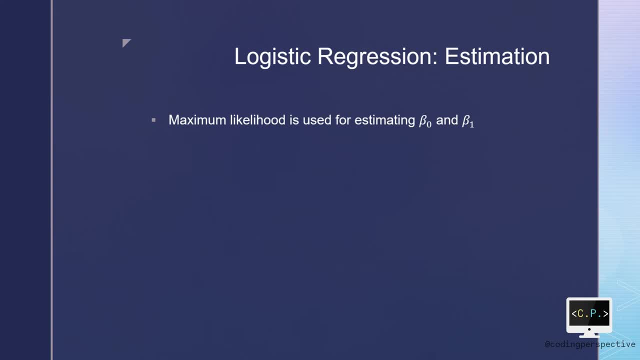 beta values that represent the data. well, The likelihood function is represented as L and it is the product of probabilities where yi's are equal to 1, and 1 minus probabilities where yj's are equal to 0. As you can see, the likelihood function is 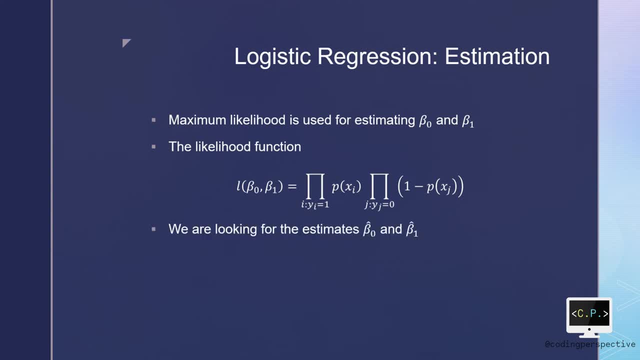 parameterized by beta0 and beta1.. We are looking for the estimates of beta0 hat and beta1 hat, which maximize the likelihood function. Assume that you have established the model and you got the estimates of the coefficients, Your model estimated beta0 as minus 8.5 and beta1 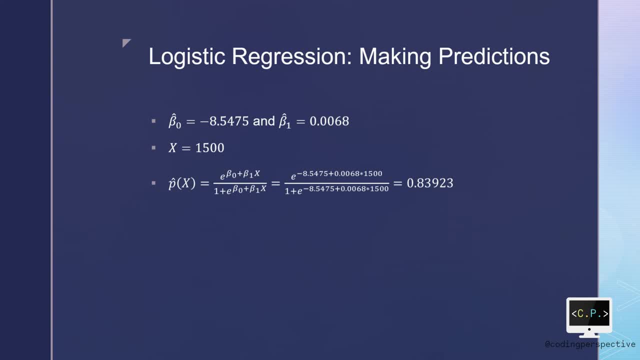 as 0.006.. Also, suppose that you have a test observation which has an x value of 15 hundredths, Then the probability of having 1 for that observation is almost 84%, which is quite high. However, if the value of x is 500, then the probability 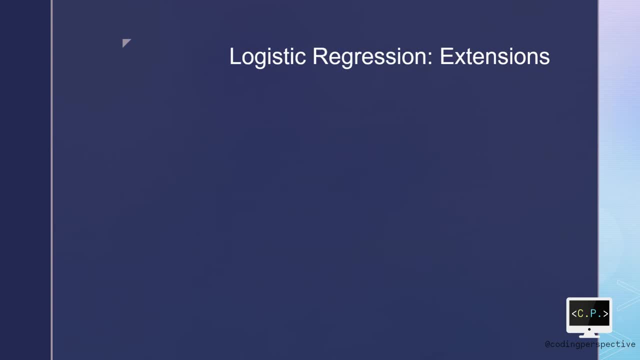 becomes less than 1%. So far, we have seen the real theory behind the logistic regression models. However, we will briefly talk about the extensions of the primitive model. The first extension would be the case where our data has more features than one feature, which would be the case for many real datasets. In that case, nothing. 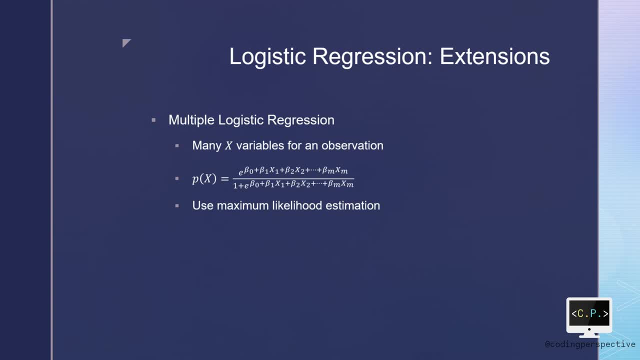 really changes in our model, except the additional terms for the logistic logistic function. For that case we have to sum over all beta coefficients and the variables x For estimating the beta coefficients. nothing changes. We will again employ the maximum likelihood method for obtaining. 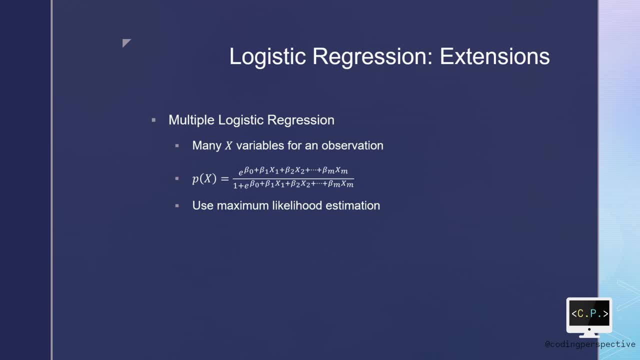 the best beta coefficients. Until now, our logistic regression models can only handle binary classification tasks. However, there are also tasks where you need to handle multiple classes. For those cases, we can extend the logistic regression model in multiple ways. Suppose that the response variable y has k different categories. The first way of 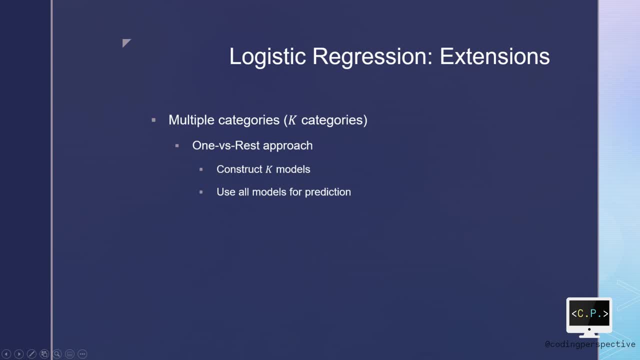 to deal with multiple classes is construct k different models. Each model is supposed to classify one category from others. In this way, you can build k different models For predicting a test observation. you need to get the probabilities from all k models and you need to select the one with the highest probability. The second way to deal with multiple